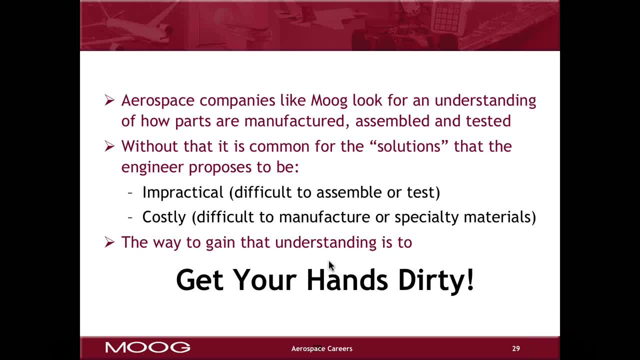 There's one other important factor for you to remember, And that's the thing that I'll say it this way: Aerospace companies like Moog look for an understanding of how the parts are made, how they're manufactured, assembled and tested. 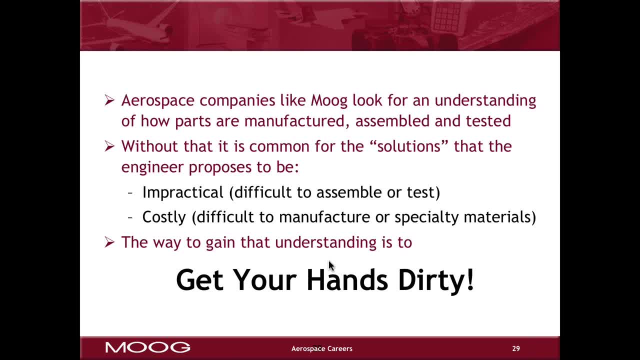 We're looking for more than a theoretical understanding of how to draw a circuit diagram or how to do a finite element analysis or how to draw a logic diagram. We're looking for young men and women who want to understand the solutions that are out there. 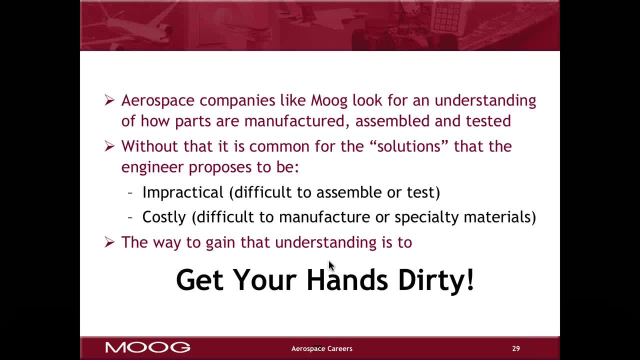 The solutions that are grounded in an understanding of how parts are made. Otherwise, it's easy for a young engineer to propose solutions that are either impractical, because you can't assemble or test them easily, or too costly, because the manufacturing methods are too costly or they use special materials that are too costly. 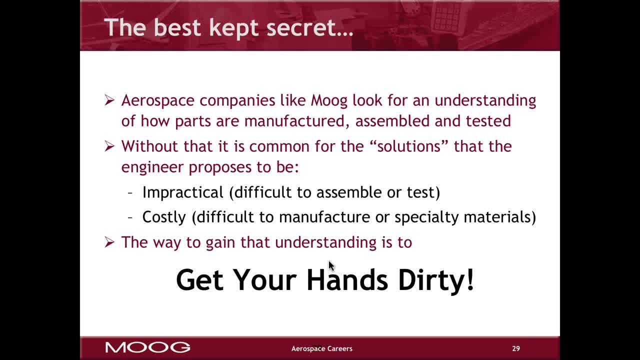 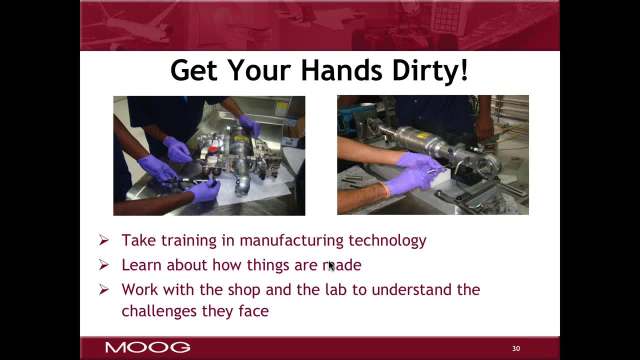 The simple way to explain that perhaps the best kept secret is the way to gain real good preparation is to get your hands dirty. Don't be afraid to get into the lab or get into the shop and actually get your hands dirty touching the parts. 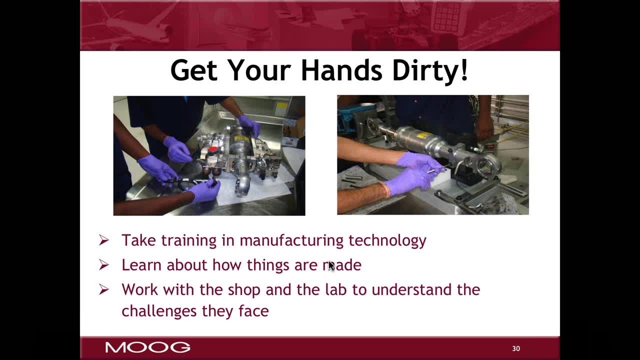 In aerospace, we believe that getting experience with the hardware is critical, and the engineer who sits at the desk with the computer and never engages with the hardware is at a big disadvantage. We'd encourage you to take training in manufacturing technology to learn how things are made. 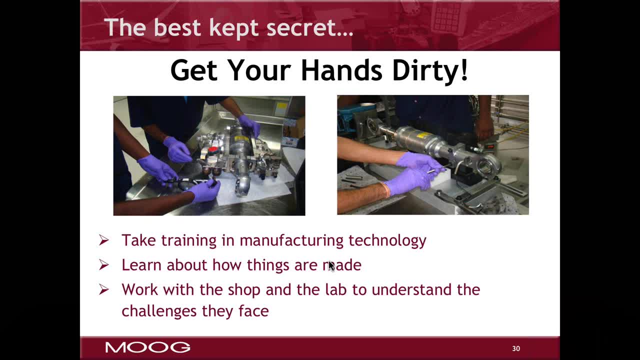 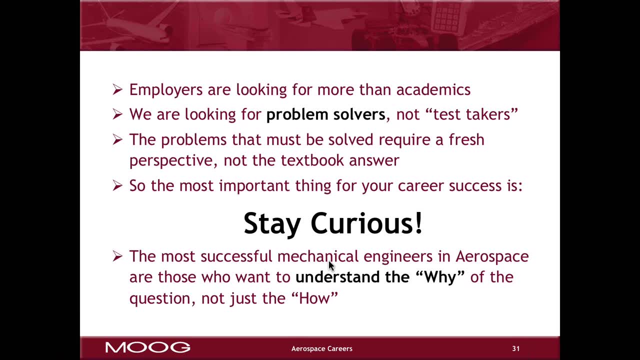 We'd encourage you to if every opportunity you get to work with the shop and the lab and understand the challenges that are faced there. If I were to summarize a lot of those thoughts and distill them down into just a few things, 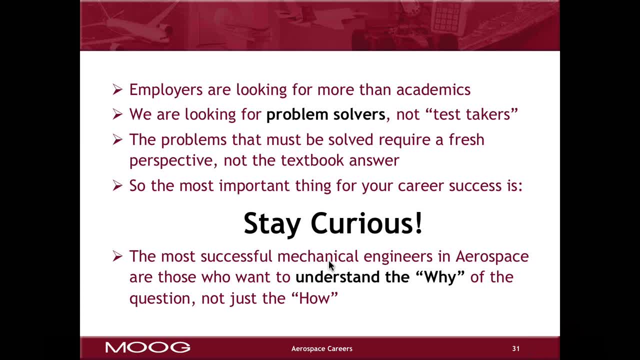 I'd say it this way: Employers are looking for more than academics. Your exams are very important And the We would expect that you'll be very good at your academic subjects And, because of the competition for joining the companies, the higher scores will actually give you a higher visibility in the recruiting process. 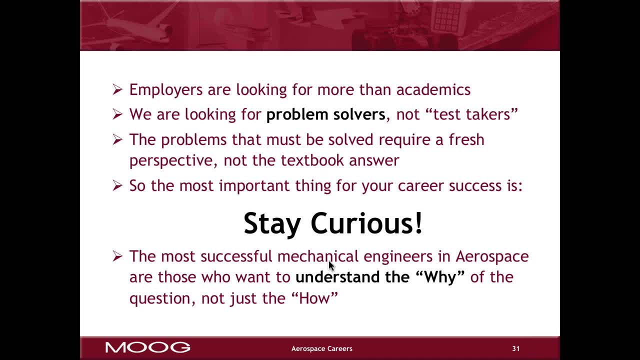 But ultimately we're looking for problem solvers, not test takers. The problems that we have to solve in aerospace require a fresh perspective, not the textbook answer. So the most important thing for your career success is to stay curious. Start with the foundations and stay curious. 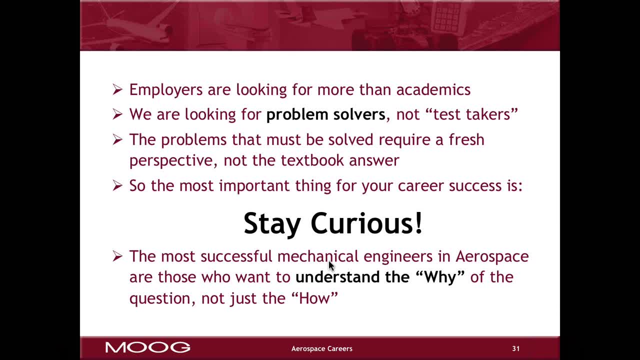 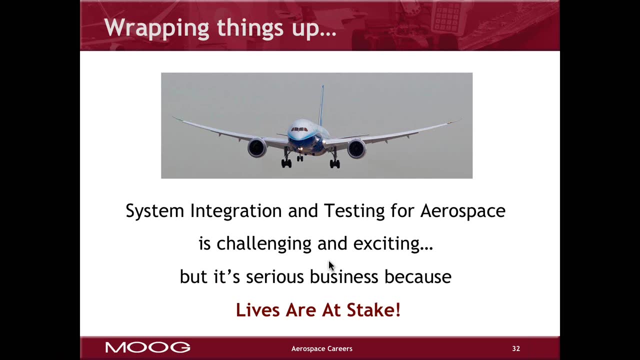 And the rest will come. The most successful mechanical engineers, electrical engineers, computer engineers in aerospace are those who want to understand the why of the question, not just the how. The most important thing Stay curious. So as we start to wrap things up here in the talk before we get to our questions, 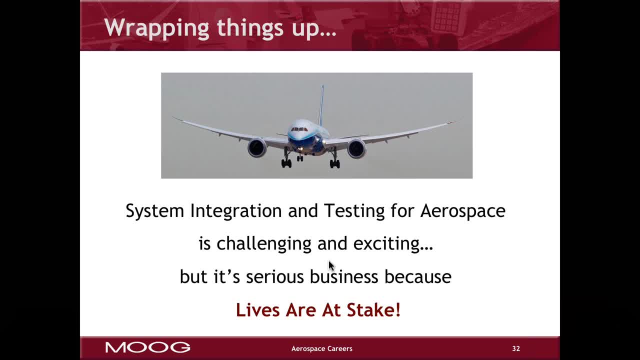 I'd like to say just a few things to remind you of where we've been. The first part I'd like to remind you is the system integration and testing domain for aerospace is challenging and it's exciting. We're working on things that fly. 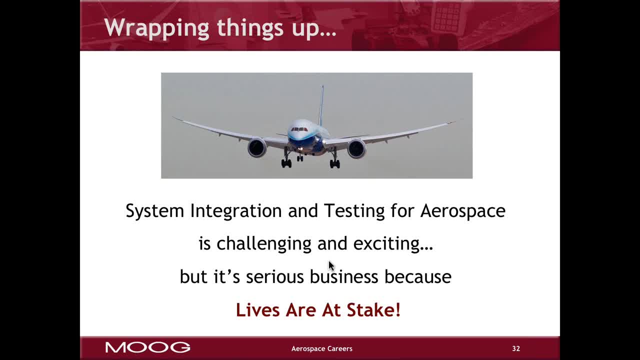 We're working on products that go to Mars. We're working on products like UAVs and fighter jet fighters, commercial aircraft, satellites. All of those are it's exciting work, But it's a serious business Because lives are at stake.